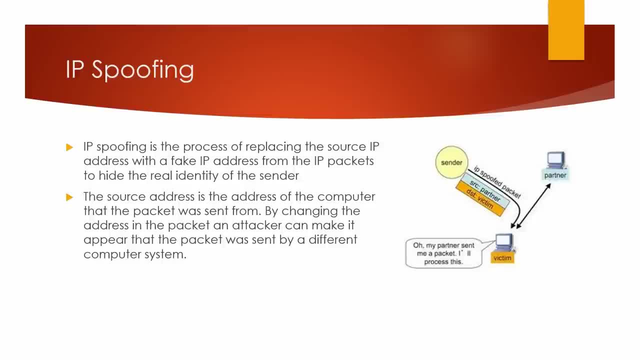 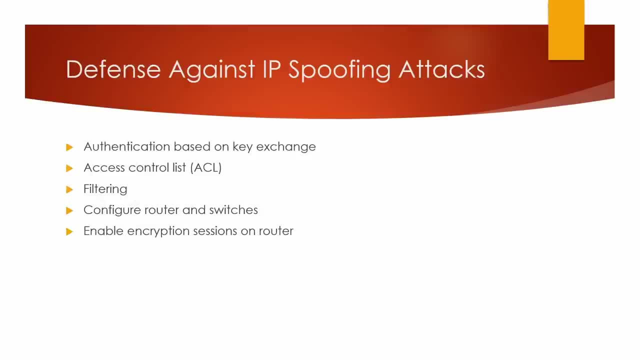 okay, I have a demo at the end of this PowerPoint and hopefully that gives you a better understanding of it. You can defend against IP spoofing attacks by using authentication based on key exchange between the machines on your network, Something like IP security, also known as IPsec. 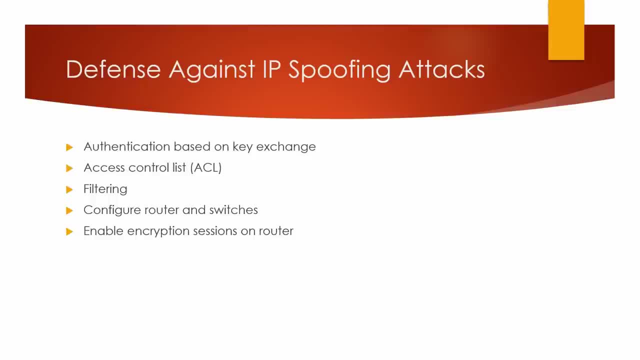 will significantly cut down on the risk of spoofing. You can use an access control list to deny private IP addresses. on your downstream interface, You can implement filtering on both inbound and outbound traffic. You can configure your routers and switches, if they support such configurations, to reject packets originating from. 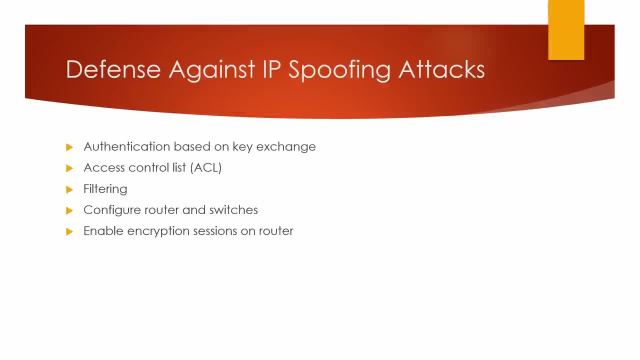 outside your local network that claim to be originating from within. Lastly, you can enable encryption sessions on your router, so that trusted hosts that are outside your network can securely communicate with your local hosts. Now then, let me give you a demo on a type of IP spoofing. 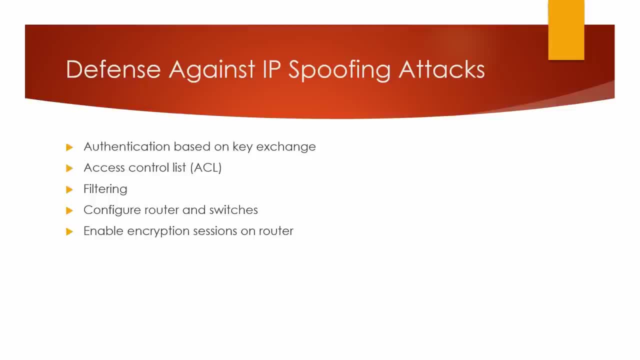 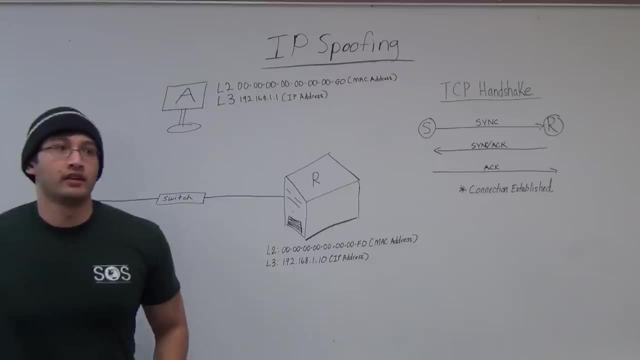 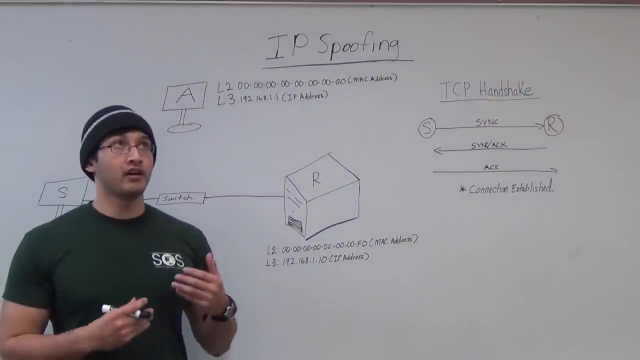 known as non-blind spoofing, in which the attacker resides on the same local area network. Hopefully, this gives you a better understanding again of IP spoofing. Alright, good day. Today we're going to cover IP spoofing. As you already know from my presentation earlier, IP spoofing involves: 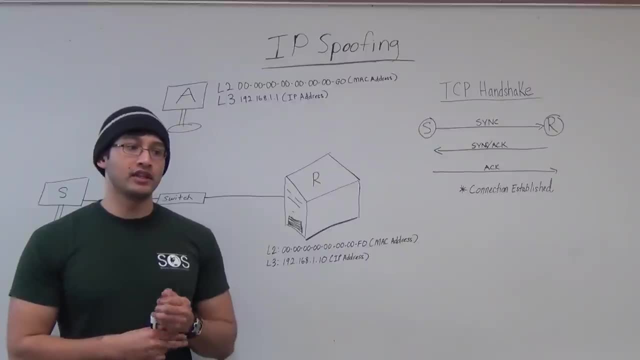 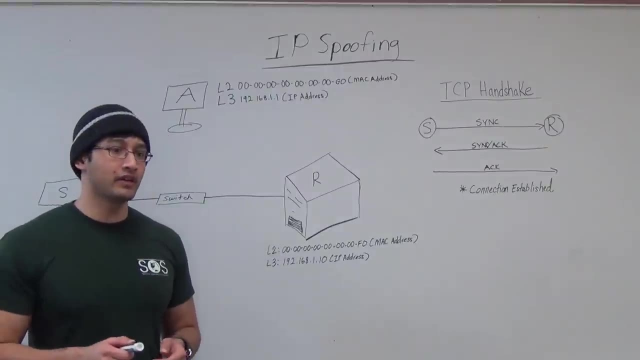 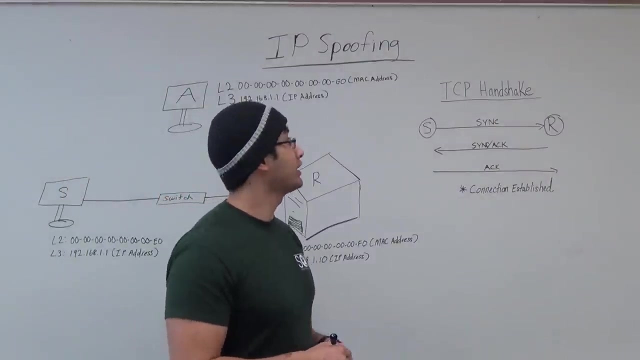 basically, an attacker steals the source IP address of the victim and pretends to be a legitimate user. So let me give you a better visual on exactly how that works. So, before we begin, I want to talk about TCP handshake, because you need to understand how. 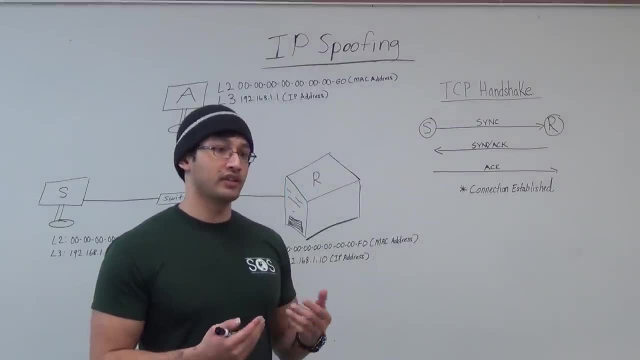 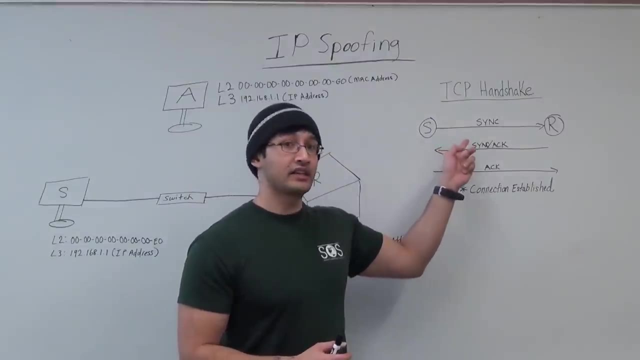 the three-way handshake works before you can understand the IP spoofing that I'm going to explain. So, first off, the sender will send a packet with a sync, as in synchronized, to the receiver. Alright, the receiver is going to receive it and respond back with a packet. 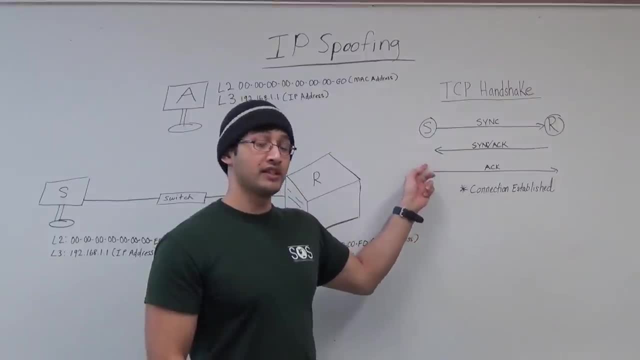 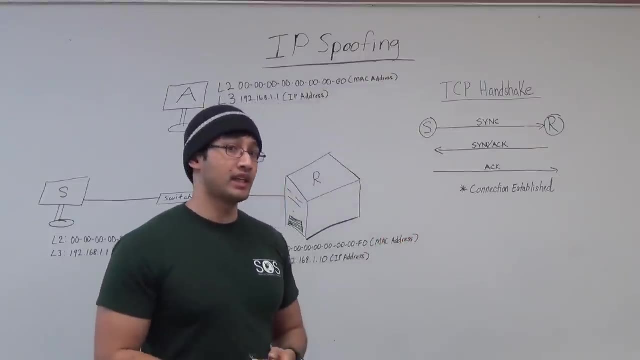 with a sync and acknowledge. Once the sender receives it, he will send an acknowledgement to the receiver. Once that all happens, they have a connection And that's what they call a three-way handshake. Now, with that, we're going to use that same thing. 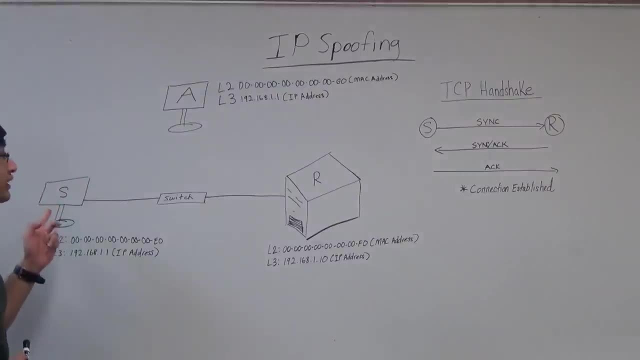 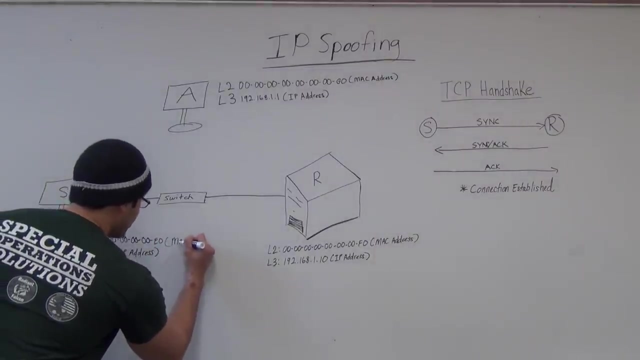 So, over here, we have the sender, we have our attacker and we have our receiver. Alright, also, we have our layer 2, which is our MAC address, and we have our layer 3, which is our IPv4 address. 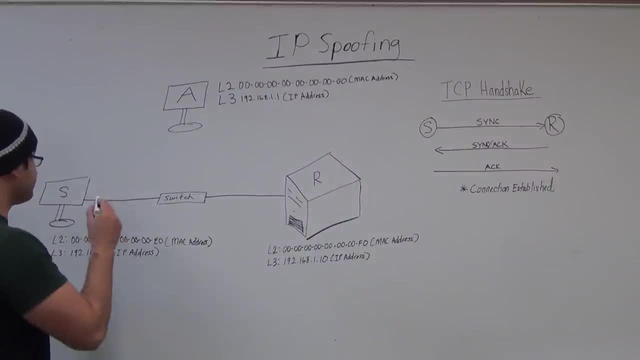 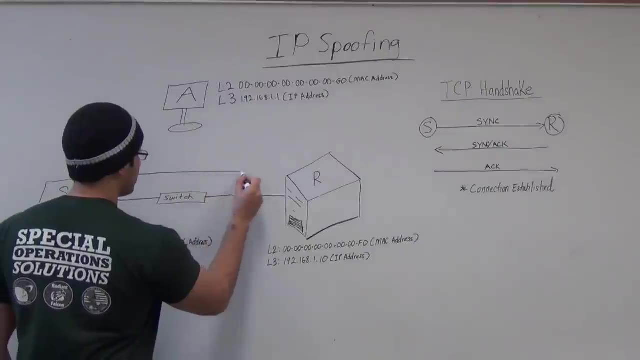 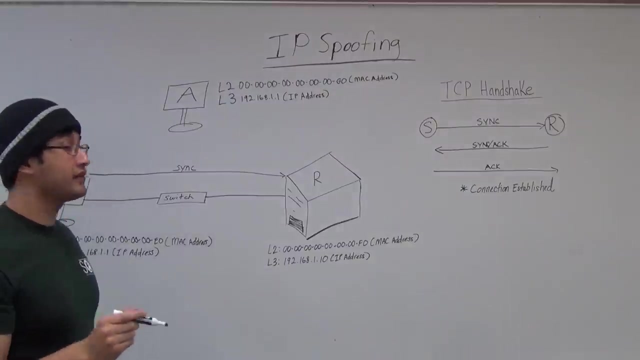 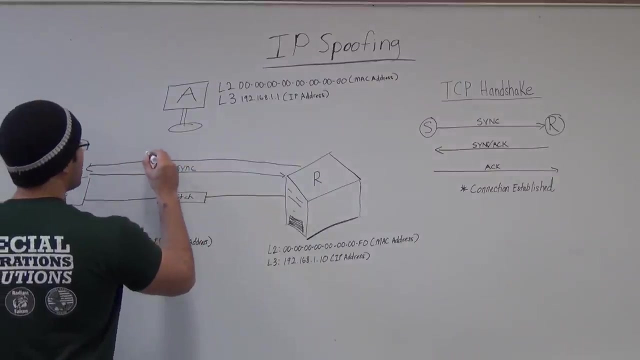 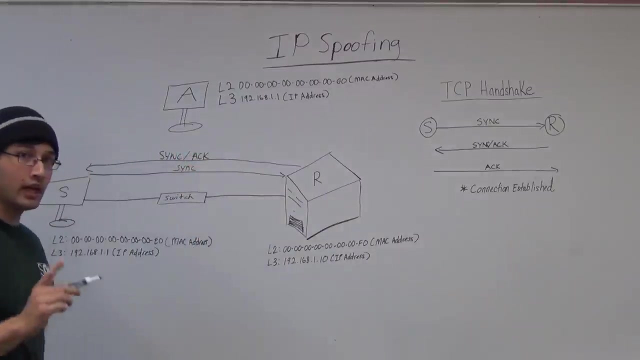 Alright. so what's going to happen is this: The sender is going to send a packet to the receiver along with the sync, as I mentioned earlier. The receiver is going to receive that packet and respond back with a packet along with the sync and acknowledge. 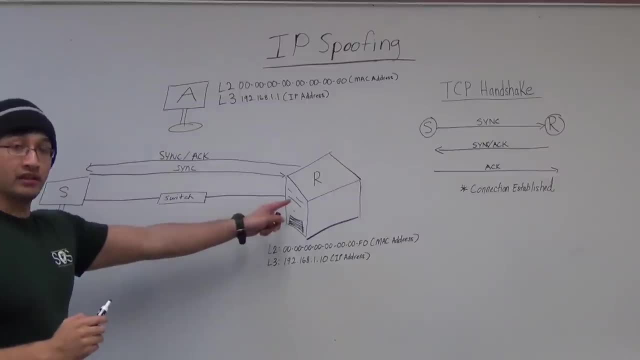 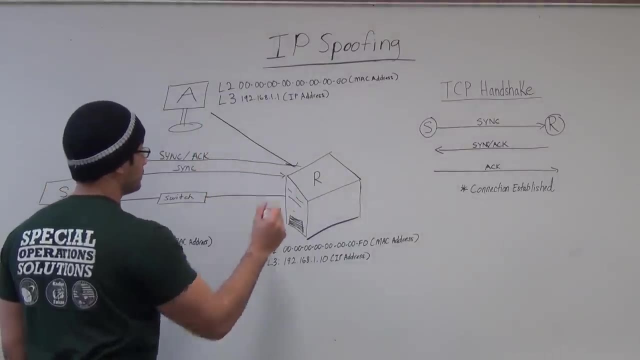 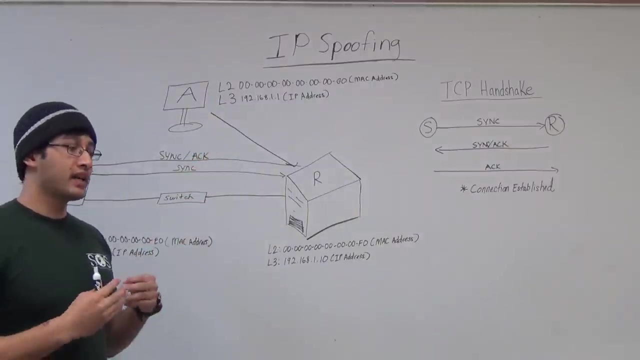 However, before the sender can send an acknowledgement to the receiver, the attacker sends it first. He does this by predicting the TCP segment number. Alright, so you need to know that inside the TCP header they have a source, they have a destination address. 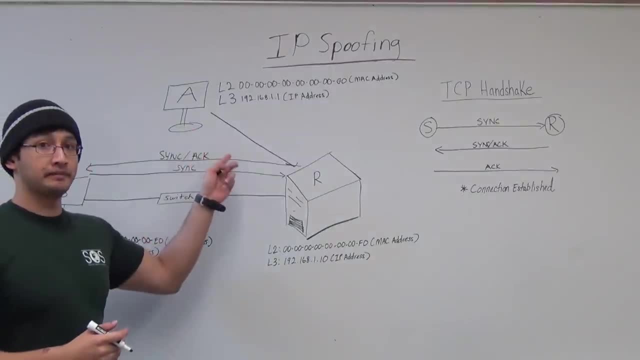 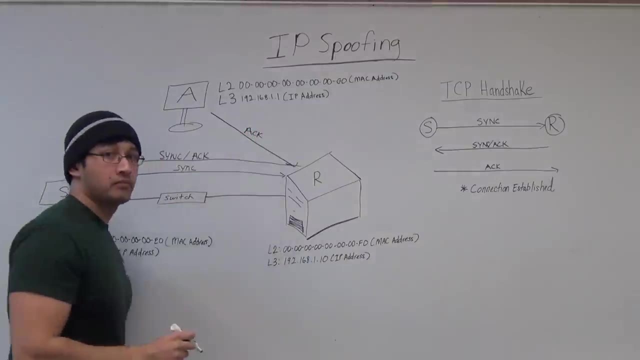 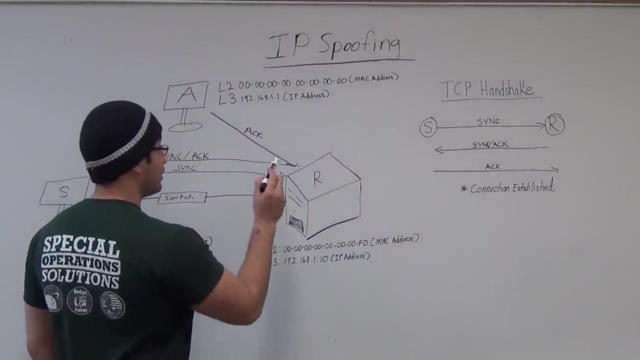 but they also have a sequence number Because he's able to predict it, he's able to send the acknowledgement before the source, before the sender. So what happens is this: The receiver is going to trust the attacker, It's going to trust that the 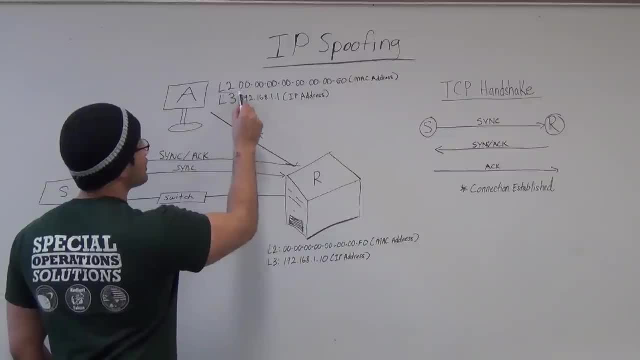 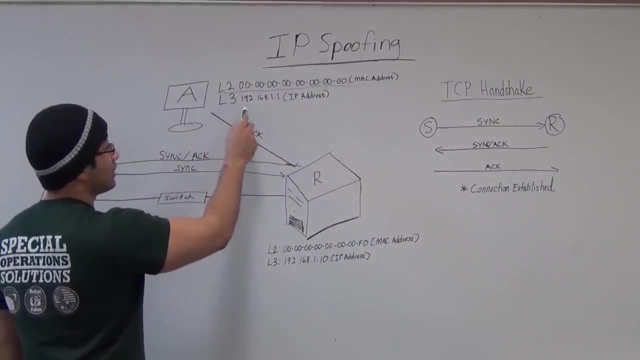 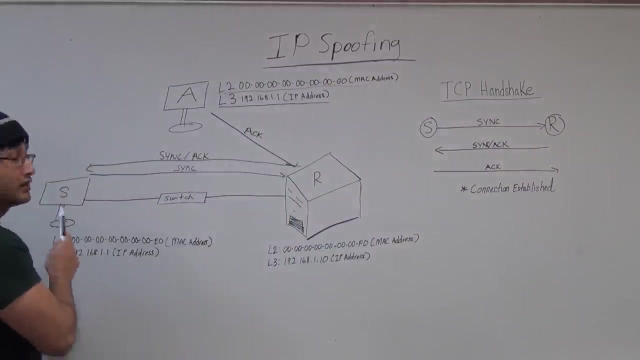 layer 2,. this MAC address, the physical address, will ensure that the packet will go to the layer 3, which is the 192.168.1.1 IPv4 address, which belongs to the sender. Again, the attacker has spoofed it. He's pretending to be the sender right now. 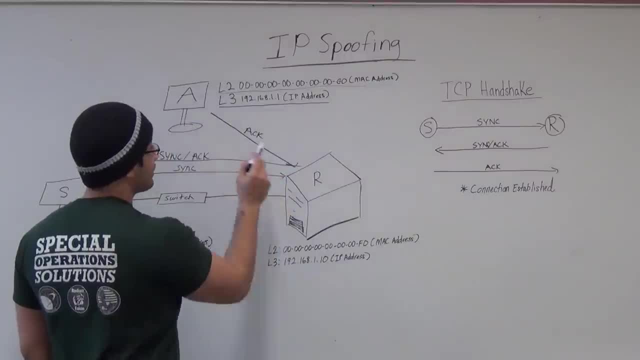 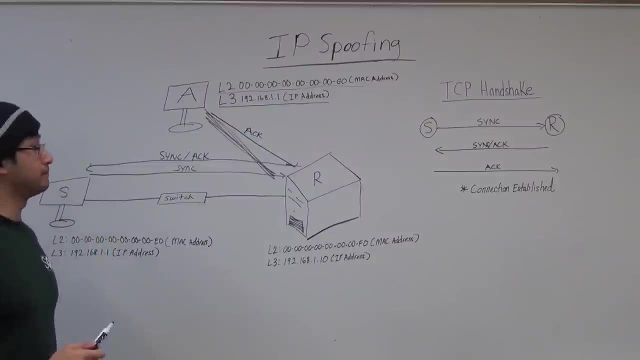 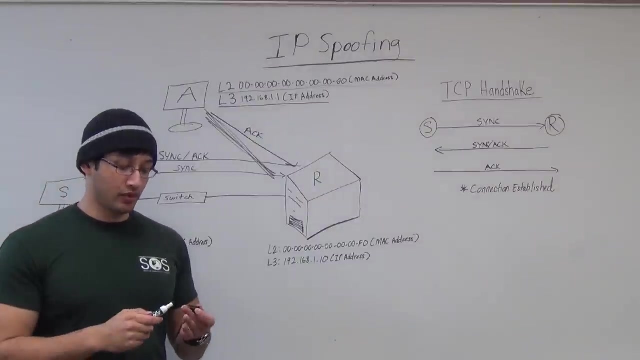 So, then, what's going to happen is communication between the attacker and receiver will be ongoing, whereas the sender will not know, And that's how IP spoofing works. Alright well, I hope that gave you a good understanding of it, If you have any more. 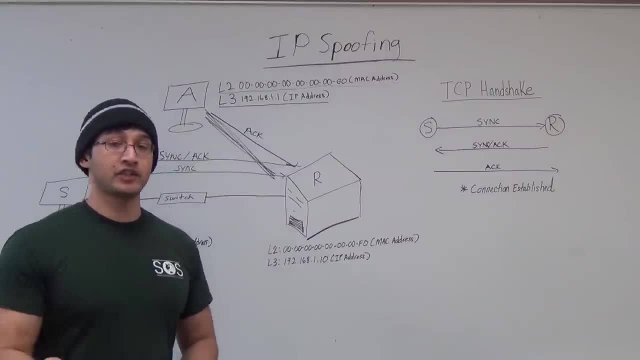 questions or want to learn more, follow my link in the instructor's note. Alright, thank you.